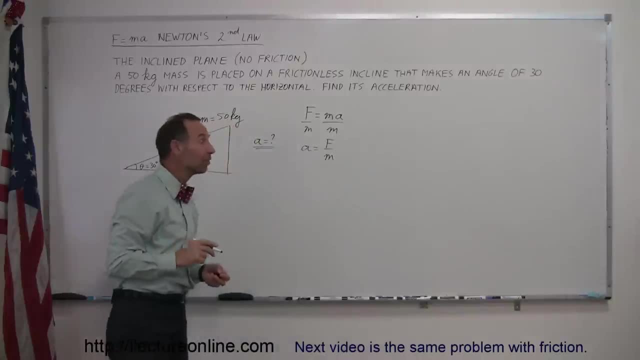 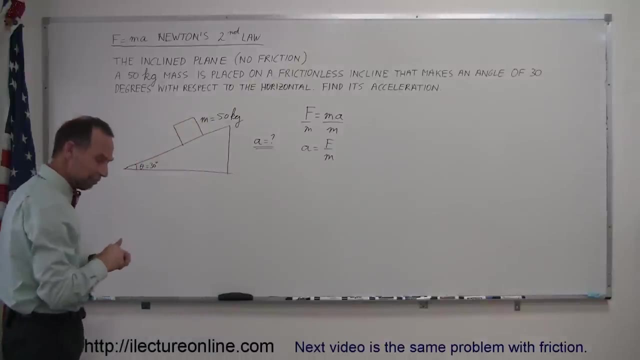 So what we need, then, is we need to find the force that acts on this object, and we divide that force by m, and we'll get the resulting acceleration. So what is the force? Well, let's figure that out by drawing the force vectors. 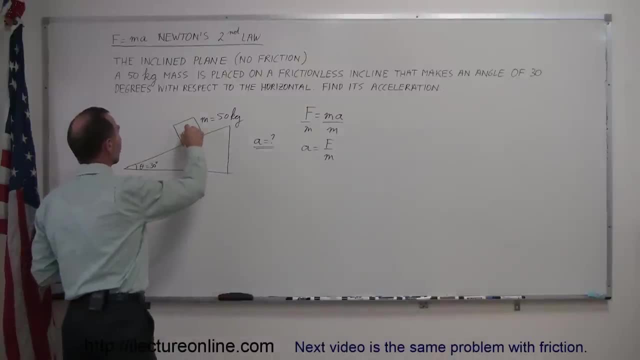 So the first one we can think of is the force of gravity pulling down on the object. So the force of gravity is equal to mg and since it's on an inclined plane, we want to divide that component of the force into its perpendicular component. 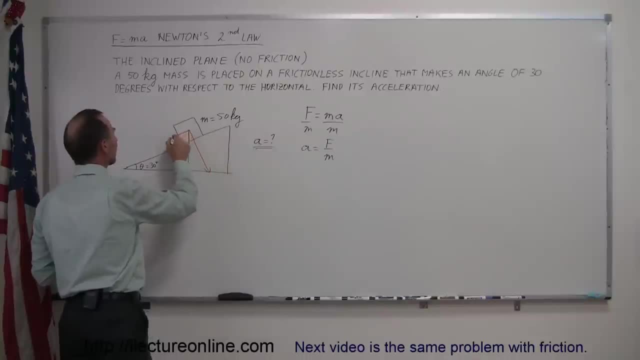 the component that's perpendicular to the inclined plane and the component that's parallel to the inclined plane. You can see that if you add this component and this component together, you'll end up with this component again, The angle between the vertical component and the component that's perpendicular to the inclined plane. 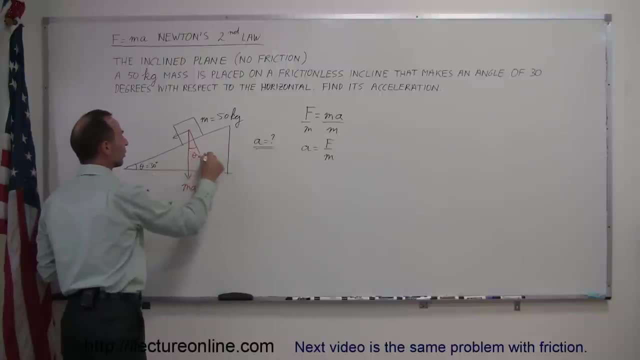 theta is the same as this angle right here, So this is also 30 degrees and therefore that makes this component equal to mg times the cosine of theta, because it's adjacent to the hypotenuse of the triangle. If you make a triangle out of that, you can see that here's the right angle. 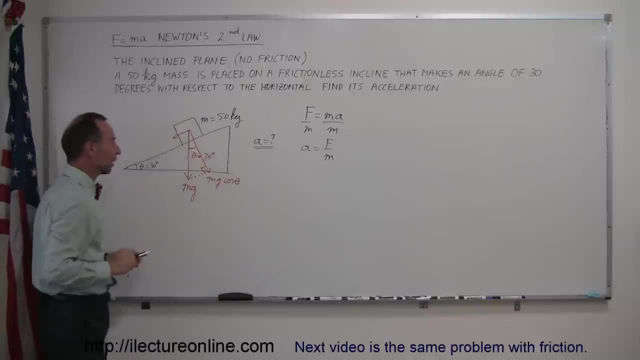 and this angle here, this side is adjacent to this angle right there. so it's mg cosine theta. That makes this component mg sine theta. Now we have one more force here, Since the object is resting on the inclined plane, pushing down the inclined plane. 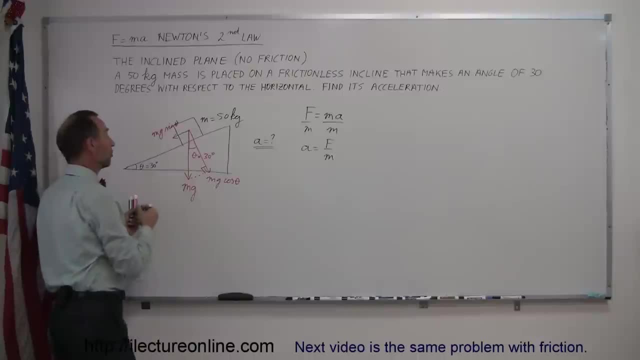 Newton's third law tells us that there's an equal and opposite force pushing back. so there'll be a force pushing back in this direction, and so that would be what we call the normal force force pushing back. Notice that these are equal and opposite in direction. 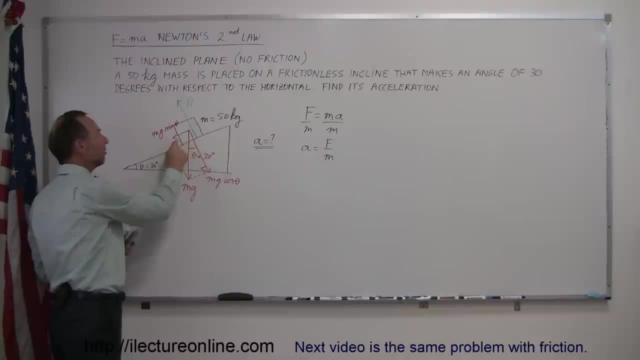 That means that those two components cancel out, and this is the only component left. This is the net force. so we could write: F net is equal to mg sine theta. It's directed down the incline and that's the force, the net force. 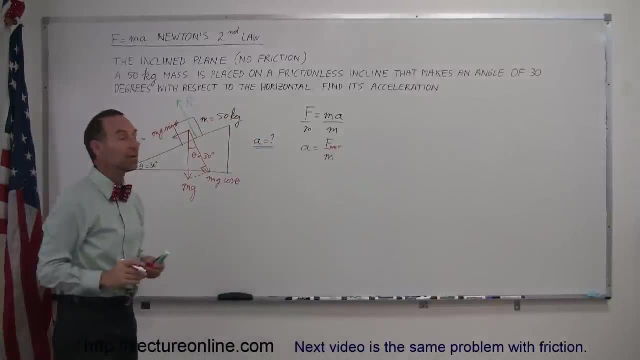 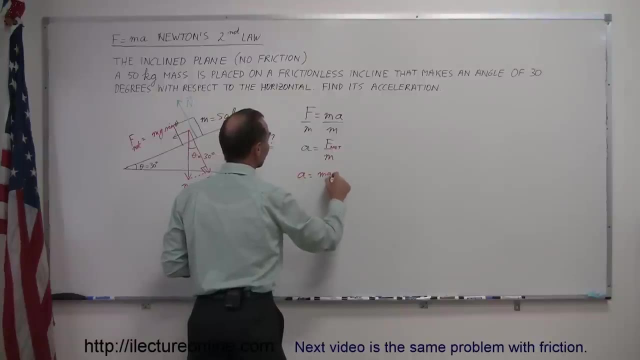 and we can call this the net force that will cause acceleration of the mass. So we can now say that the acceleration A is equal to the net force, which is mg times the sine of theta divided by the mass of the object. M Notice that the masses cancel out.